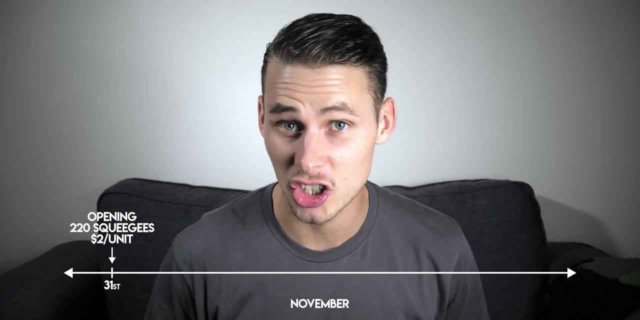 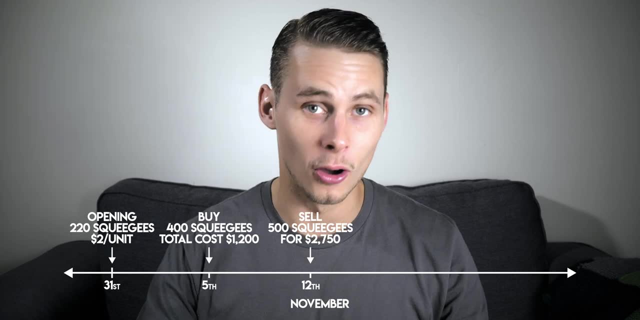 squidgees in your inventory. These cost you two dollars each. On November 5th you buy another 400 squidgees for one thousand two hundred dollars, and a few days later, on November 12th, you sell 500 squidgees for $200. 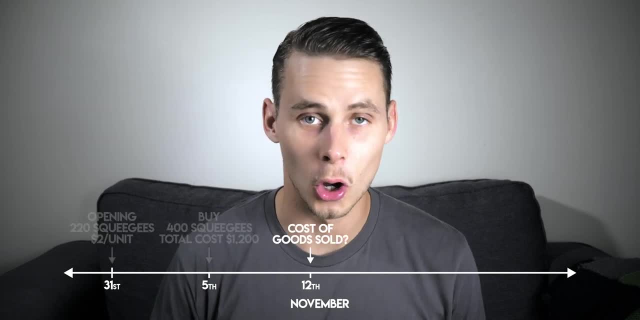 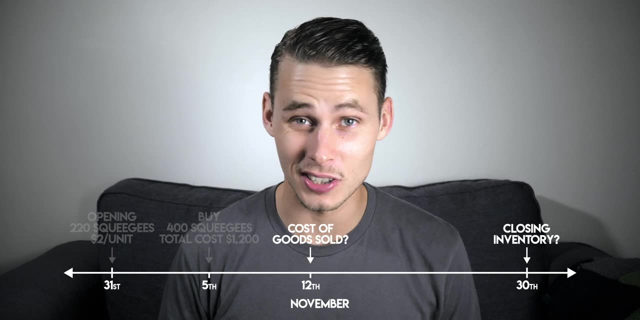 Two thousand seven hundred and fifty dollars. What's your cost of goods sold and closing inventory for November, assuming that you're using the LIFO cost flow assumption? Last in, first out. It's time for some steps. We'll go through them now, but you can also get them on my inventory. 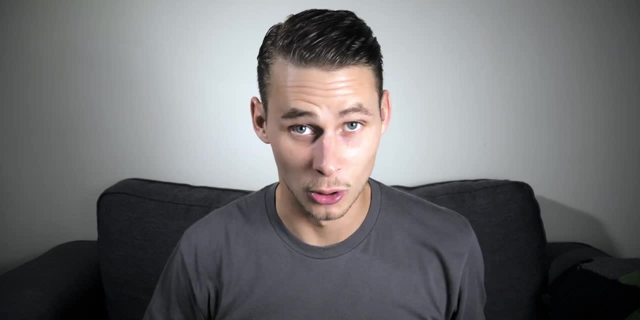 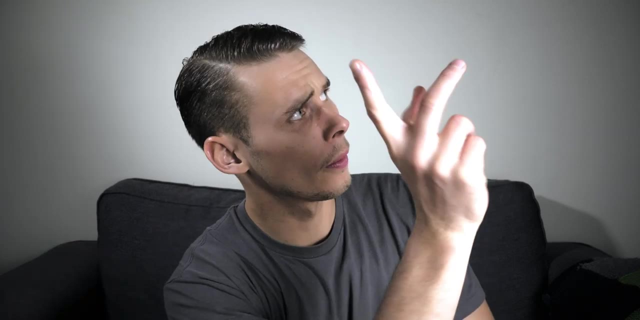 cost flow assumptions- cheat sheet. If you're finding these accounting tutorials at all helpful and you'd like to help support the channel, then the best way you can do that is by buying one of my cheat sheets. You can find the link up here and down below, as usual. 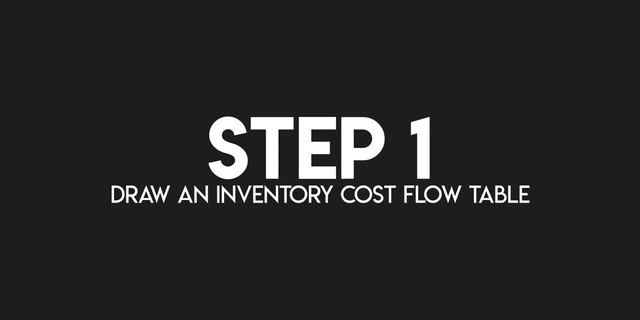 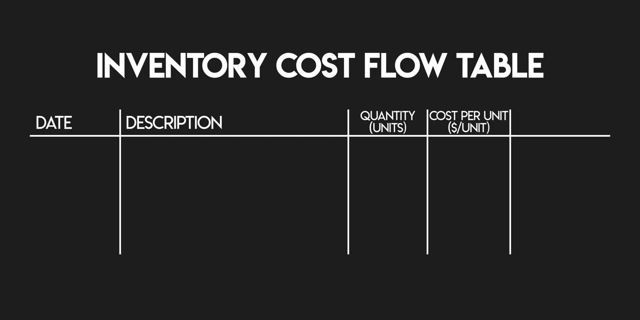 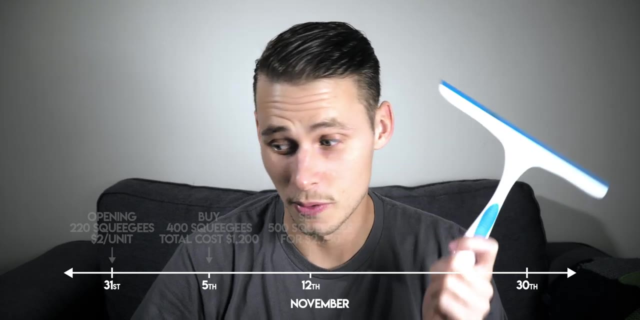 Step one: Draw an inventory cost flow table. This is a table made up of five columns: Date, description, quantity, cost per unit and total cost. Step two: Enter what you know. What do we know? We know that you began November with 220 squidgees, which cost you two dollars per. 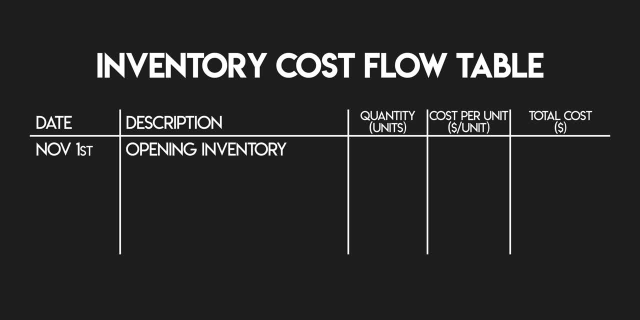 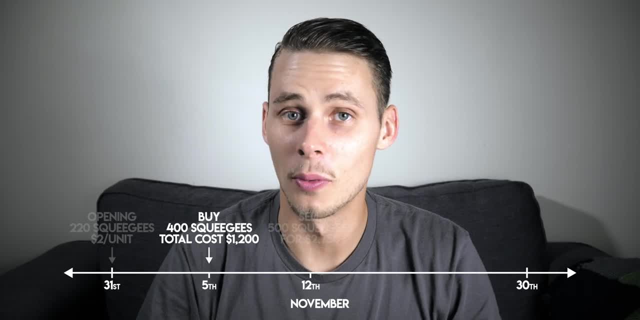 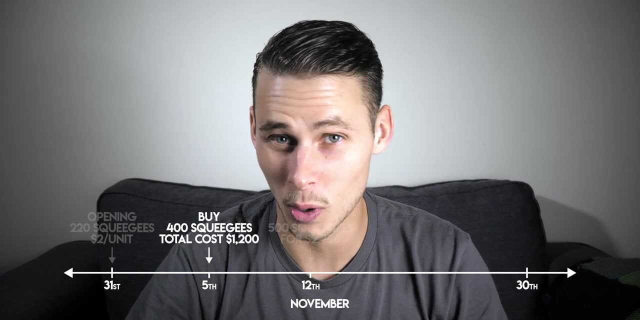 unit. So at the start of November you had an opening inventory of 220 units, which cost you two dollars each. On November 5th you went and bought another 400 squidgees, costing you one thousand two hundred dollars in total. This belongs in the table as well. On November 5th, 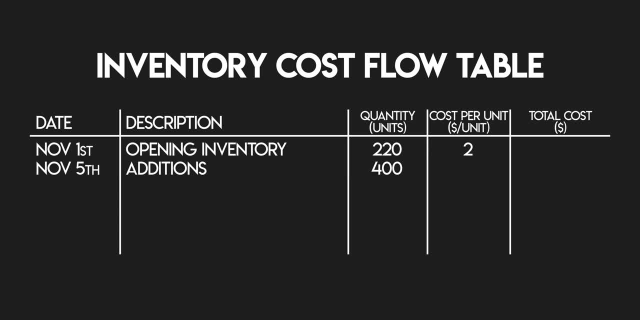 you added 400 units to your inventory, which came to one thousand two hundred dollars. In the inventory cost flow tables, you want to leave blank rows beneath each addition or sale. This gives you some room to put your goods available for sale, which is the subtotal of the 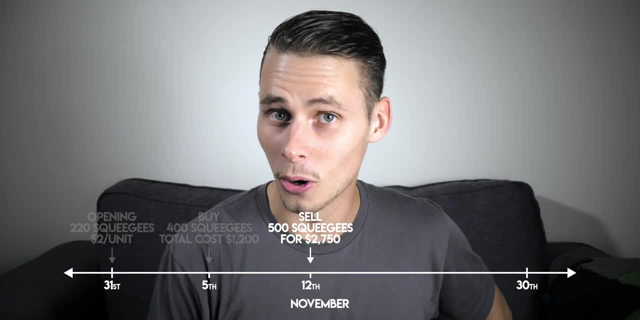 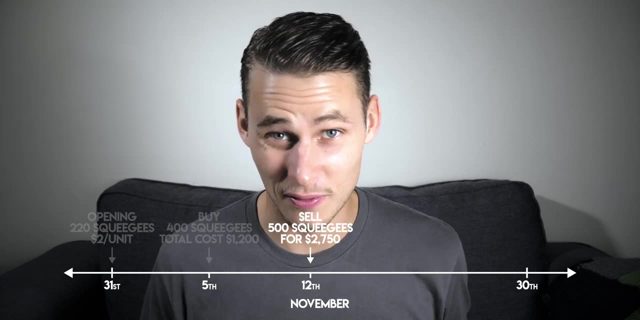 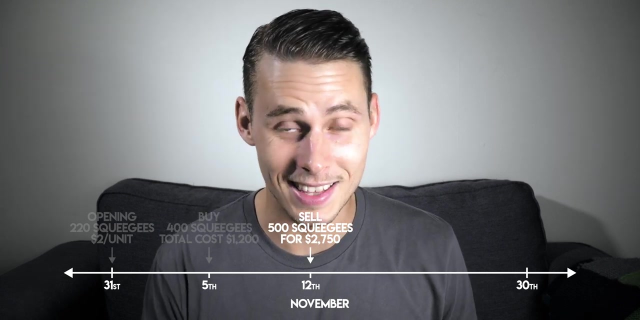 goods directly above it. On November 12th, you sold 500 squidgees for two thousand seven hundred and fifty dollars. Now be careful here. This two thousand seven hundred and fifty dollars is the revenue that you've earned, not the cost of goods sold that you've incurred, So it doesn't belong. 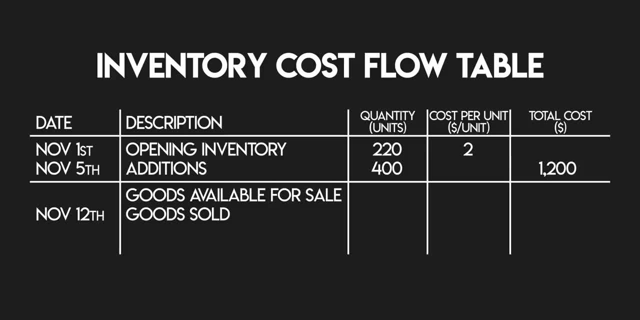 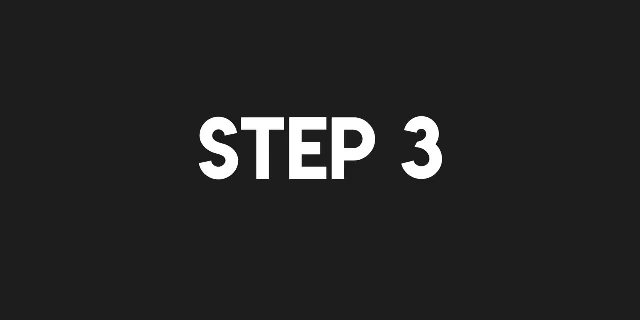 in the inventory cost flow table. So on November 12th you sold 500 units and that's all we know about this transaction. We'll need to work out your total cost of goods sold later. We're also going to calculate your closing inventory on November 30th. Right step three. 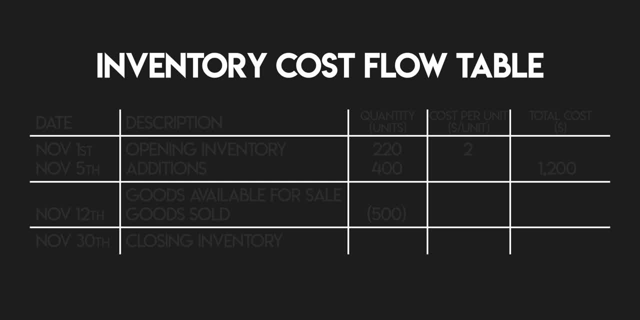 We need to fill in the blanks. We'll begin by calculating the total cost of your opening inventory. You kicked off the month with 220 units, which cost you two dollars per unit. 220 multiplied by two dollars is 440 dollars. Next we'll work out the cost per unit of your additions. 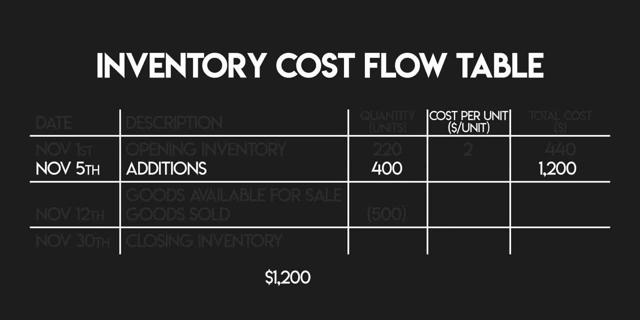 One thousand two hundred dollars in total. One thousand two hundred dollars divided by four hundred units is three dollars per unit. Now we can take some subtotals to work out your goods available for sale. 220 plus 400 is 620 units available for sale And 440 plus 1200 is one. 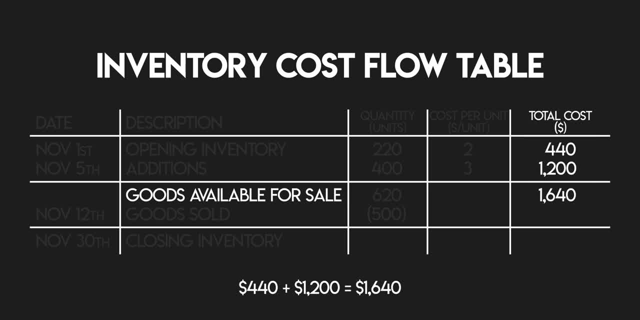 thousand six hundred and forty dollars Your total cost of goods available for sale. When using the LIFO or FIFO methods, you can ignore the cost per unit of your goods available for sale, goods sold and closing inventory, So we can move on and calculate your total cost of goods sold. 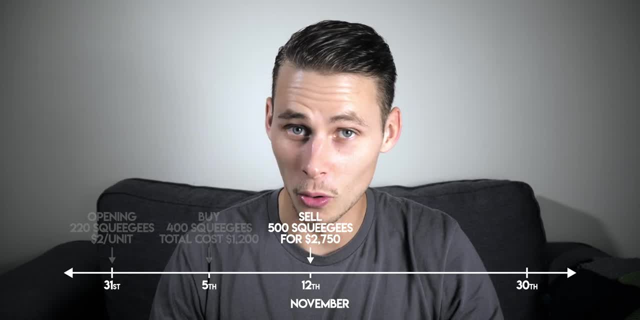 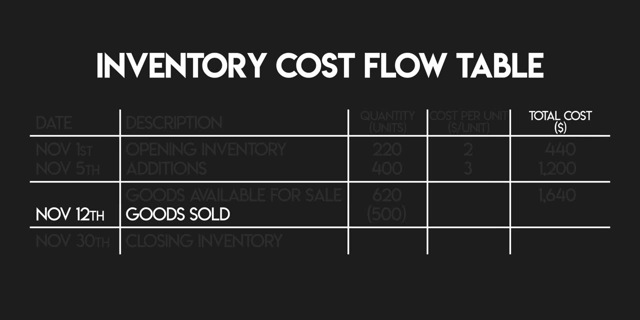 You sold 500 units, but what was the cost of goods sold that you incurred in this transaction? Remember LIFO means last in, first out. The last squidgies you bought were your additions of 400 units, but you still need to sell another 100 units to reach 500.. The next hundred units? 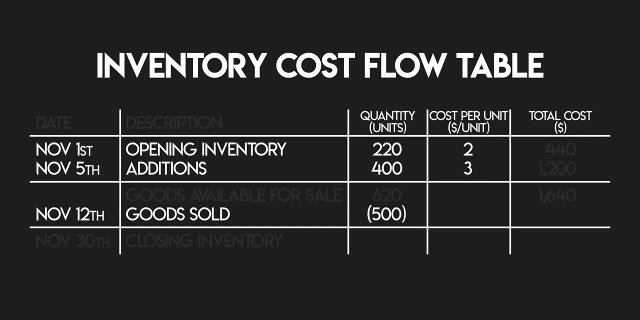 come from your opening inventory, which cost you two dollars per unit. So let's work this out: 400 units multiplied by three dollars is one thousand two hundred dollars, And 100 units multiplied by two dollars is two hundred dollars. One thousand two hundred plus two hundred is one thousand four. 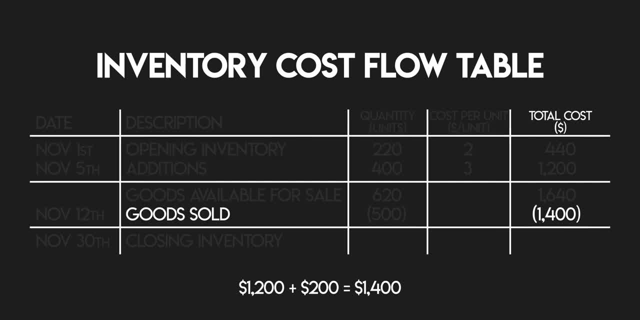 hundred dollars. This is your total cost of goods. We'll see you next time. Bye. total cost of goods sold. great, that's the tough bit out of the way. now let's find out your closing inventory on November 30th. to do that we need to take some totals. 620 minus 500 gives you 120 units. 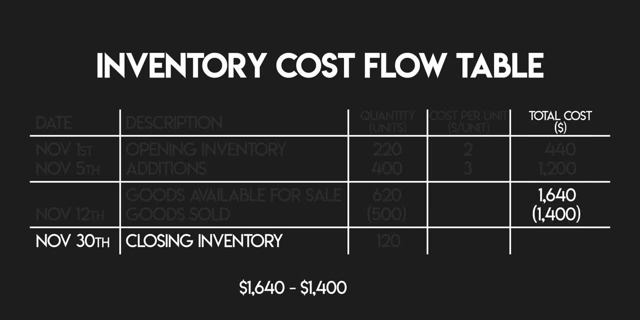 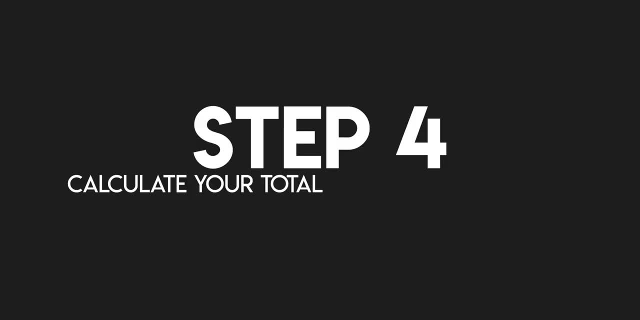 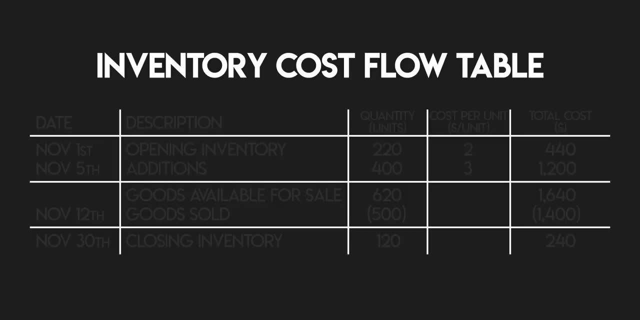 and 1640 minus 1400 gives you 240 dollars. all right. step four: calculate your total cost of goods sold and your closing inventory. your total cost of goods sold for the month can be calculated by adding up your cost of goods sold for every sale that you've made. in this example, you only 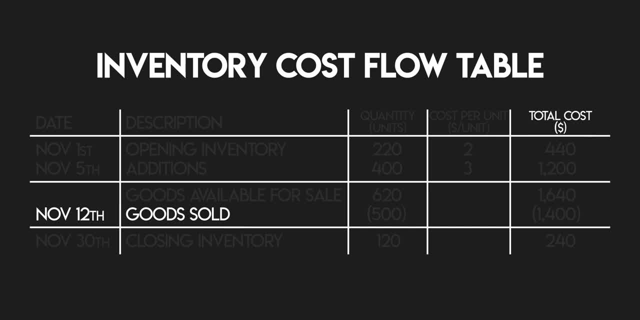 made one sale. so your total cost of goods sold for November is one thousand four hundred dollars and the total cost of your closing inventory is two hundred and forty dollars. but you can use these same four steps to solve any inventory cost problem. now let's have another look at the inventory calculation. why would you choose LIFO over? 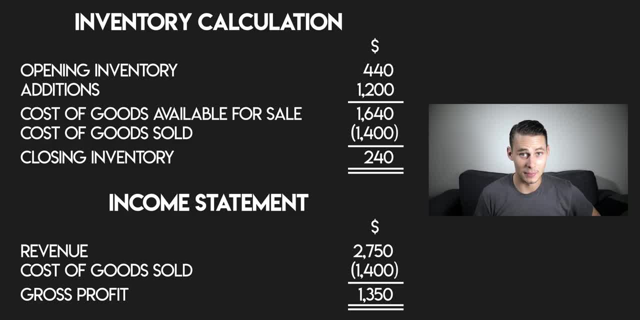 the other inventory cost flow assumptions. this method allows you to match your current revenues against your most recent cost of goods, so your gross profit reflects your business's current performance. however, when prices are rising during times of inflation, your most recent cost of goods are also your highest, which gives you a higher cost of goods sold. remember those squidgees in 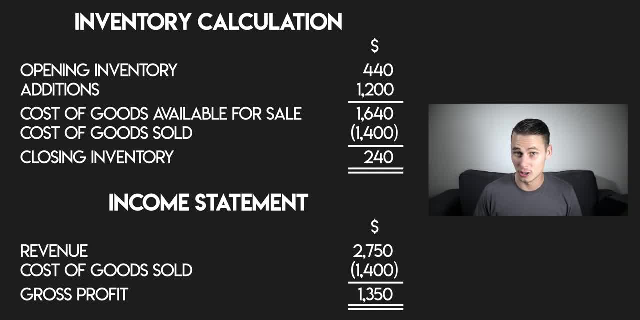 the example below are the cost of goods sold and the cost of goods sold in the example below are the cost of goods sold and the cost of goods sold. in the example below are the cost of goods sold. in the example went from costing two dollars per unit to three dollars per unit. this gives you a 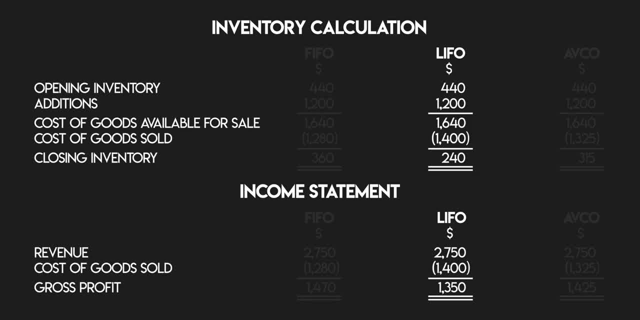 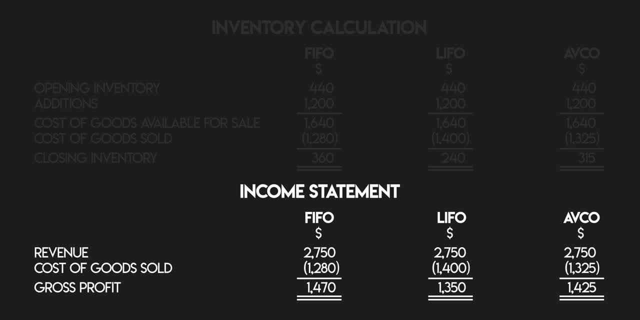 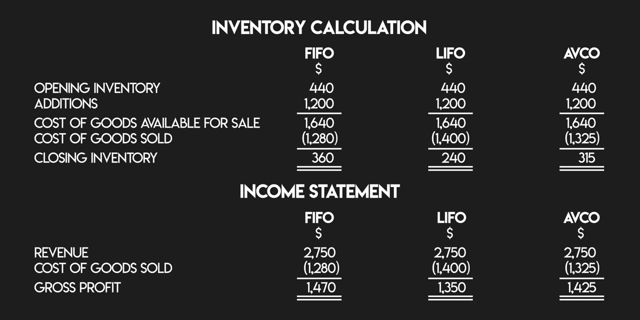 lower gross profit. so when we compare your results using LIFO against the FIFO and AVCO methods, your gross profit under LIFO comes in the lowest. but as a business owner, this can be a good thing. businesses are charged tax on their profits, so lower profits means lower taxes, which can free. 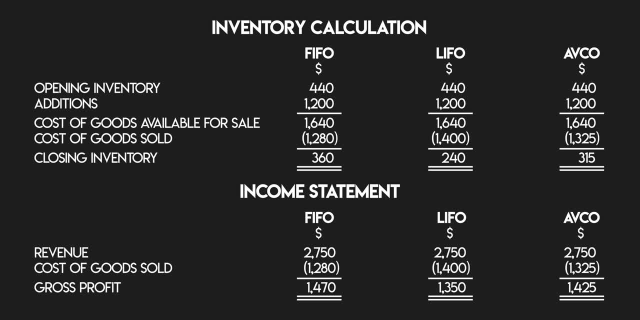 up more cash for you to use in other areas of your business, at least in the short term. but be careful: last in, first out is not allowed under IFRS. so if you follow international financial reporting standards, then you'll need to use first in, first out or the average cost method instead. 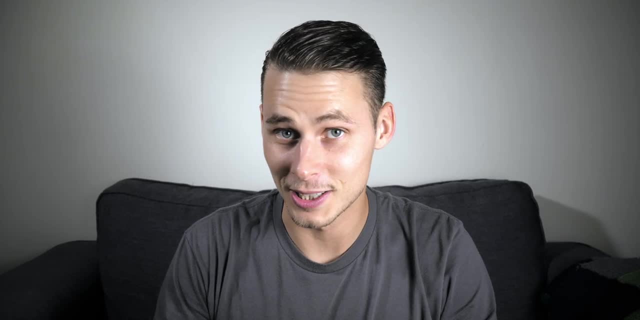 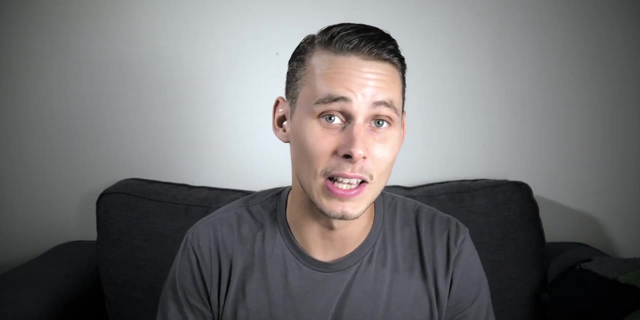 next time we'll cover the average cost method. remember to click subscribe if you'd like to see that. i made a FIFO video last week as well, so if you missed it, it's in this playlist over here, and if you're interested in buying the cheat sheet, you can find that over here as well. it's been a pleasure, as always, see you in the next video. see you next time.